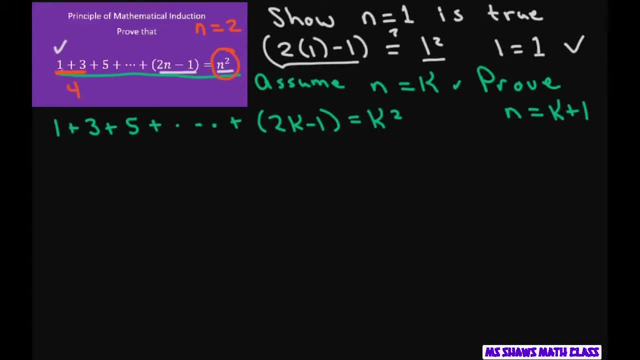 So 1 plus 3 is 4.. If I plug in 3,, I get 3 squared, which is 9, and that should be the sum of the first three terms. So 4 plus 5 is 9.. So that's what this means. 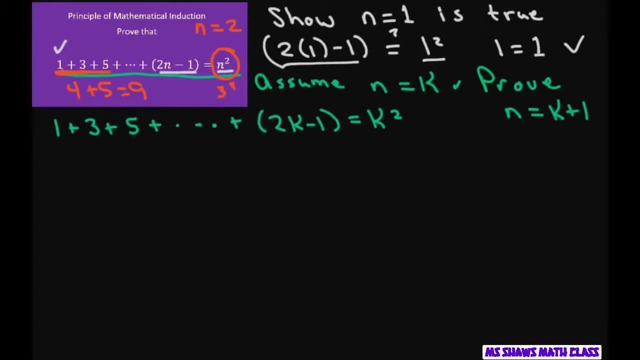 We want to prove that it works for every single time you do the next term. So what we want to do is take our k line here and plug in k plus 1.. The first step is: just remember this. Copy this part down, Just copy exactly what you have. 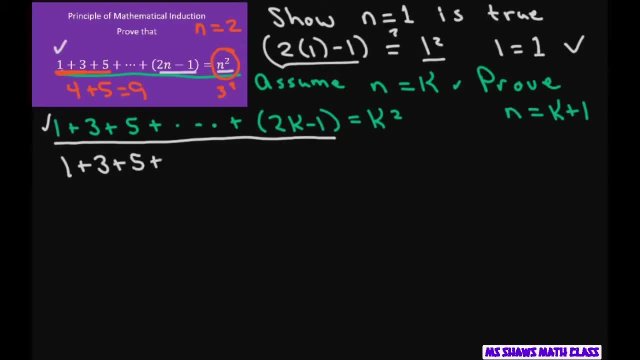 1 plus 3 plus 5 plus dot dot, dot plus 2k minus 1.. All right, I'm going to put that in parentheses, If you want. all right, and the next term? what would be the next term? 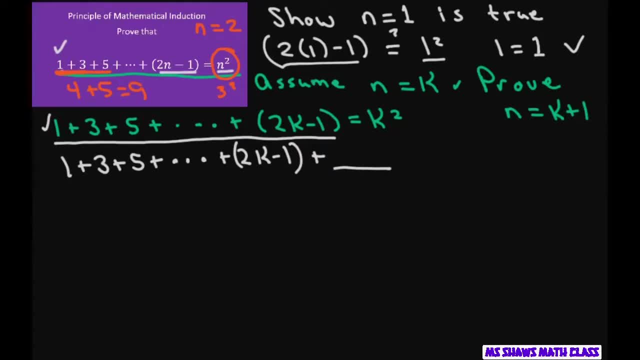 And so what you do here is you take the previous term and everywhere there's a k, you plug in k plus 1.. So I took this k right here and plugged in k plus 1.. Now, simplifying this, we get 2k plus 2 minus 1.. 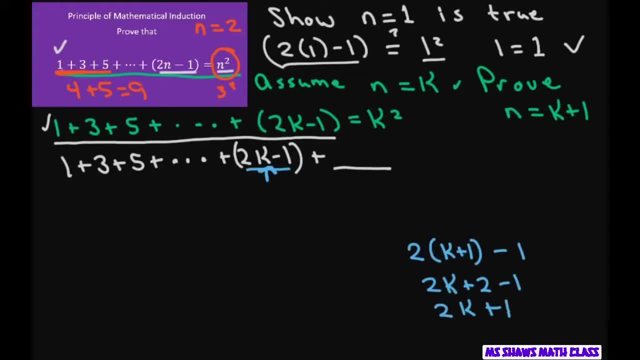 And that gives you 2k plus 1.. So 2k plus 1.. Now that's one way to do it. The other way to do it is notice that on arithmetic sequences these are linear terms, So this right here is linear. 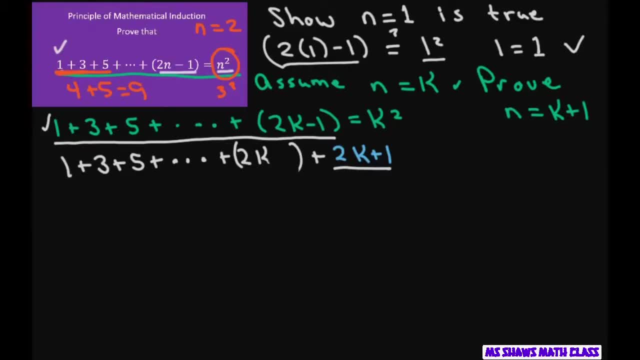 Let me write this back. Oops, All right, This is. your slope is 2.. So when the slope is 2, all you have to do is you have to plug in k plus 1. And then you have to do is add this number to this number. 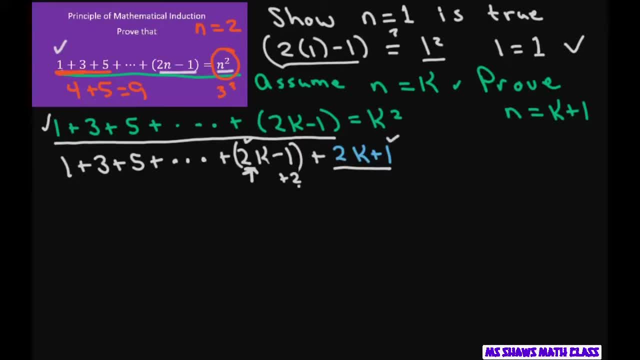 So negative, 1 plus 2 is 1.. And the next one would be 2k plus and you add 2, 3.. The next one would be 2k plus 5, and so forth, Because you just keep adding the slope for the arithmetic part. 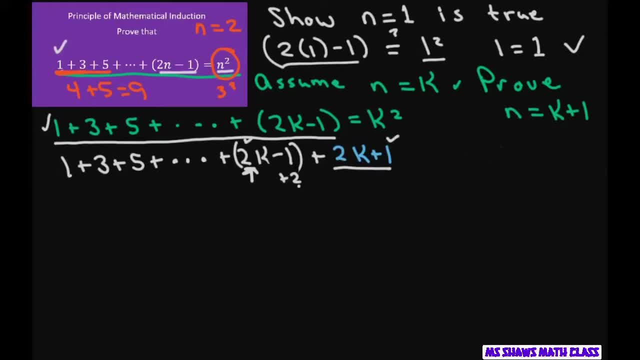 All right. Well, now that we did that, you can do it either way. We're going to write equals. Now, everywhere there's a k, We're going to put k plus 1.. So here's our k. So put k plus 1 on this side.